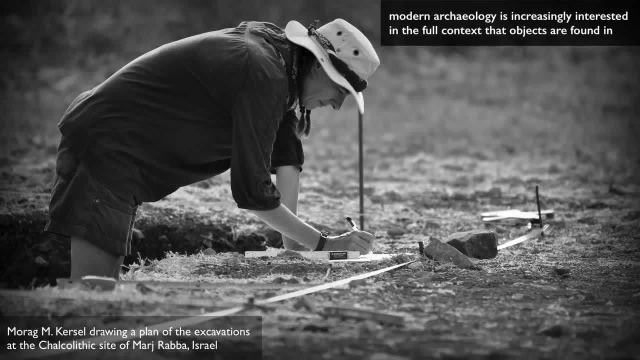 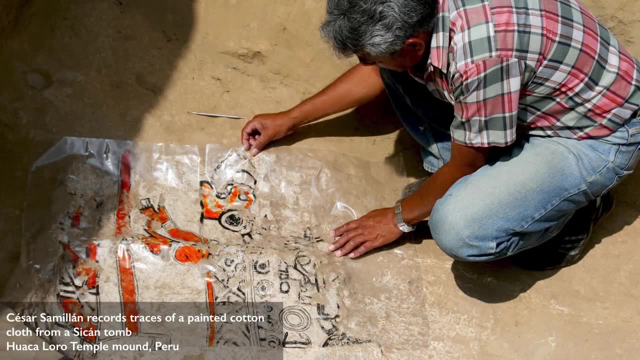 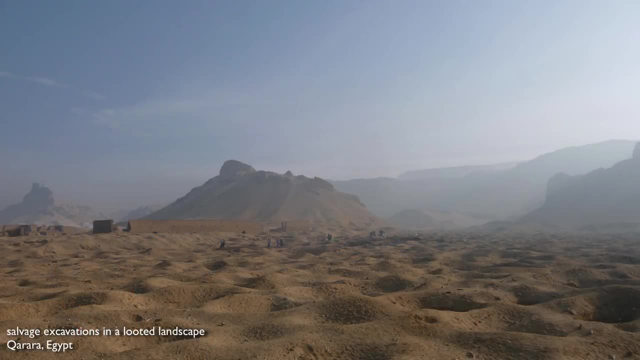 As a discipline. in the 21st century, archaeologists have come to the point where not only are they interested in the discovery and the conservation of the object, but they're also committed to the preservation of its contextual information. Often, archaeological sites are looted, and when that happens we lose so much context. 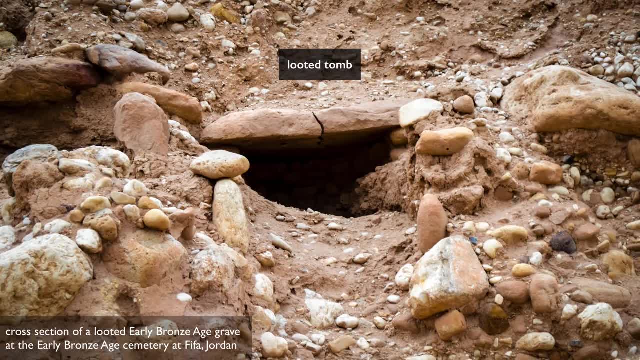 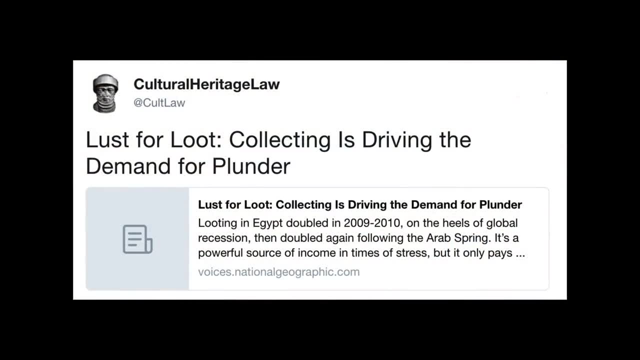 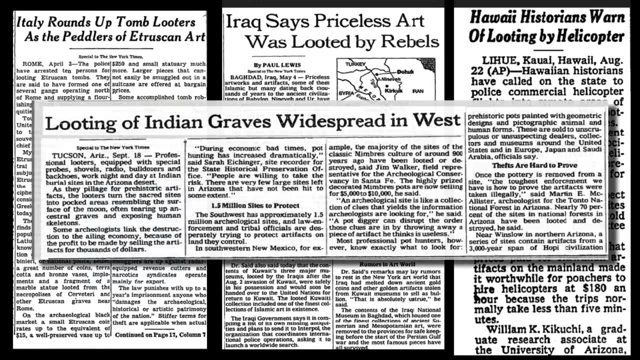 Objects are looted so that people can live and eat in parts of the world that are deeply impoverished, So there's often a sense that it's the collector at fault. It's the demand for these objects that are the problem. The looting of archaeological sites that's happening in the world today tends to be motivated by concerns. 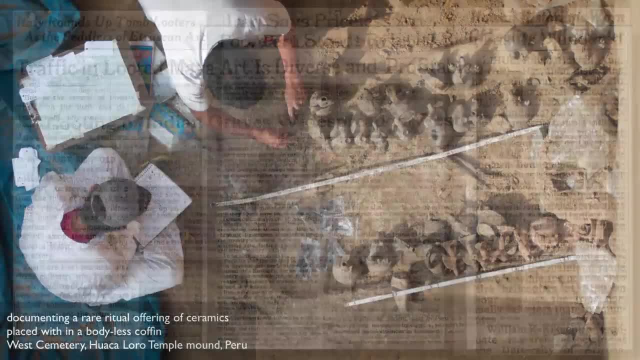 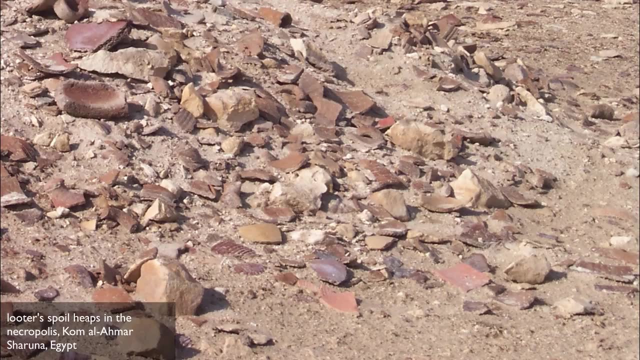 that are different from those of archaeology, in that the archaeological sites that are looted are different from the archaeological. exploration of a site tends to be slow and methodical, And looting tends to happen along a different and much quicker timeline in order to acquire extract objects. 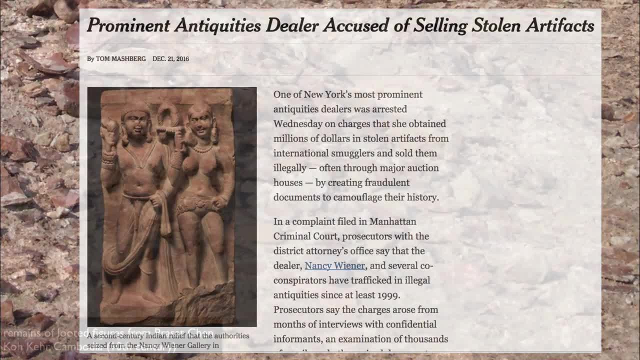 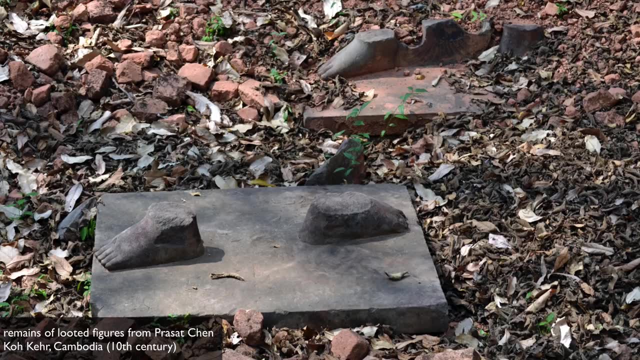 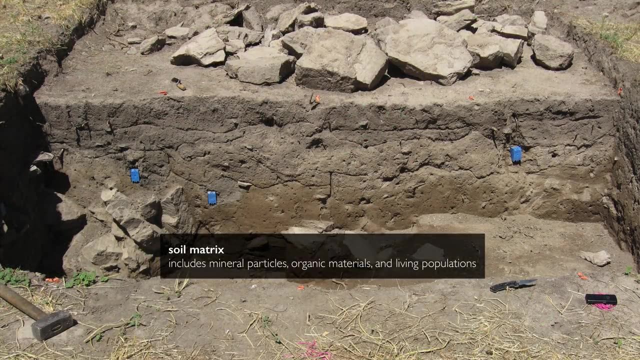 that the black market has a taste for. It often means a serious disruption of whatever the archaeological context is in the pursuit of whatever objects are desired, And often the things that are not objects per se, like the soil matrix. this helps tell the contextual story of that place. 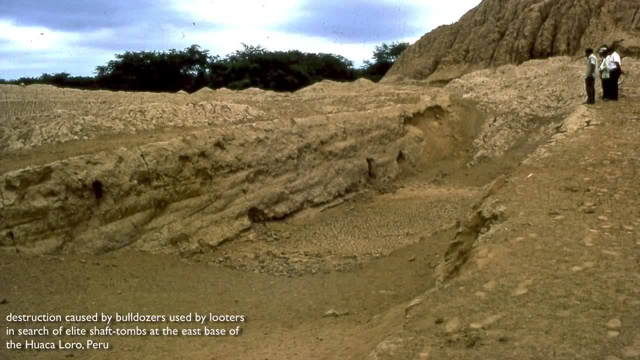 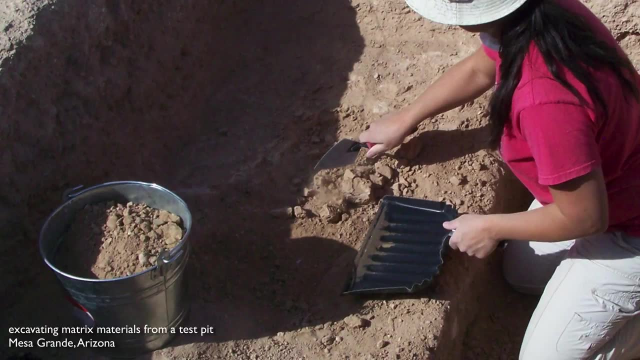 And once those are destroyed or seriously disrupted, there's no recovering them. So what can we learn from the soil matrix? We can increasingly learn more from dirt than ever before. We can even understand things about elements in human diet by looking at mineral traces in human remains. 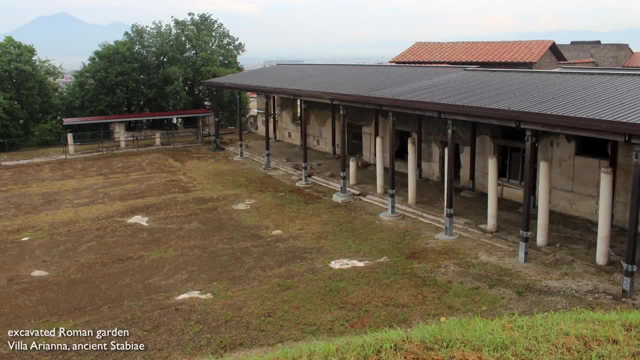 We can do garden archaeology and learn what people were growing, not just to eat but to decorate the outside of their homes, And this is an example of why contextual information is so vital. So if we privilege the object, we're losing so much. 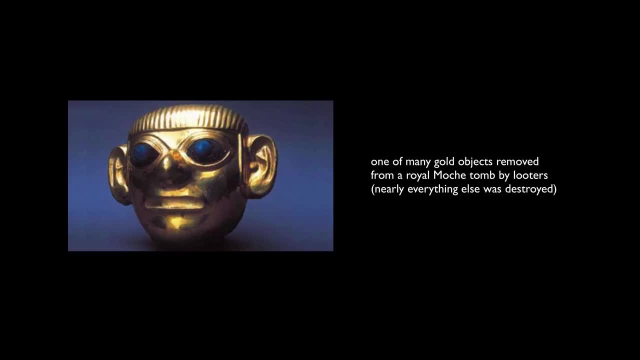 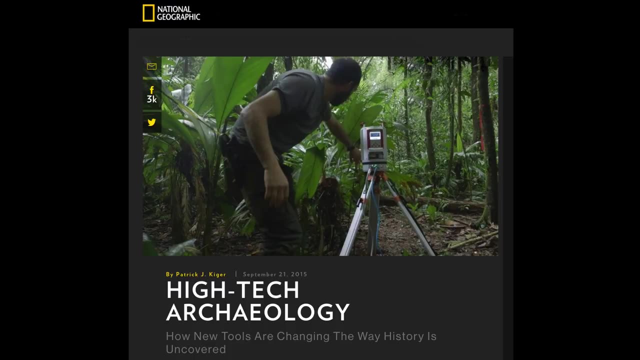 Especially if we're privileging the objects that collectors are most interested in. If we focus only on the object, we are going to miss most of the story, And these days there's so many tools for archaeologists to accurately record an archaeological site. 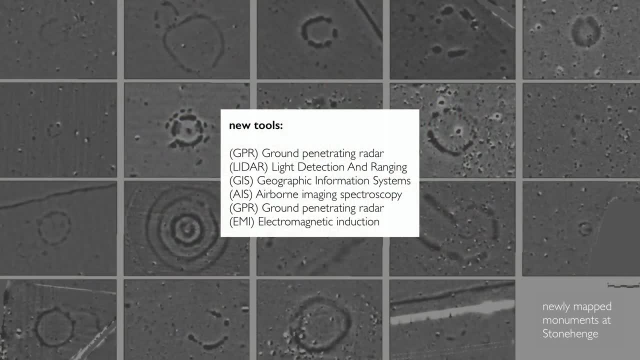 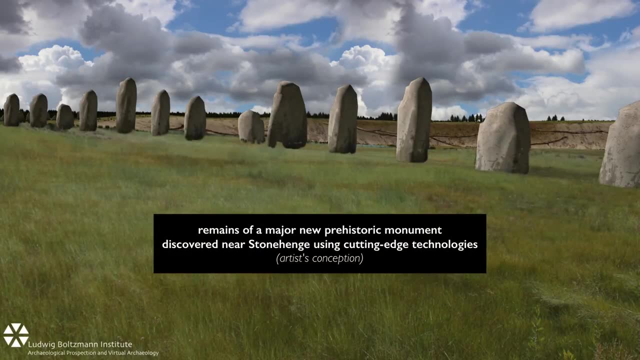 Computer-aided technology has really revolutionized archaeological fieldwork. It has not only made things more accurate, but it has also enabled us to collect more data than ever before, Such that we may even be collecting data now that scholars in the future may still be able to analyze further than we can. 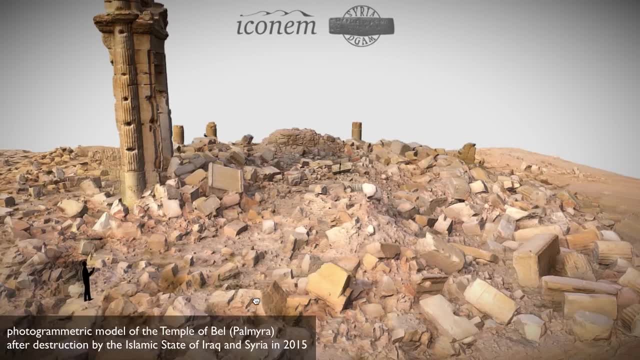 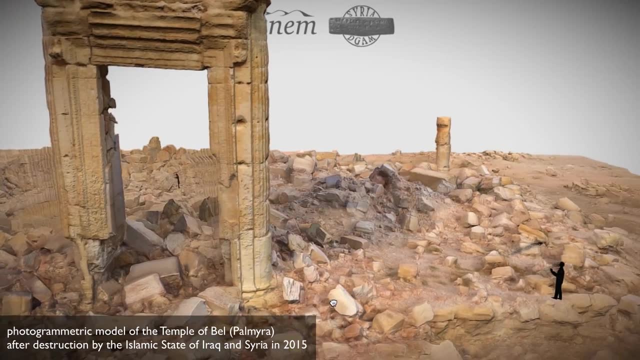 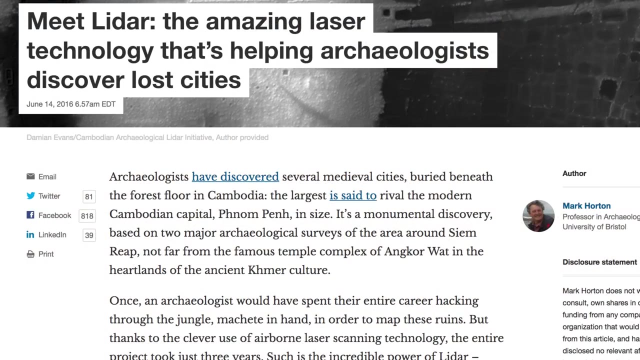 And I can even use photogrammetry to recreate that object digitally in three dimensions. Those photo models can then allow someone who was not present at the excavation to virtually experience that object or a grouping of objects in their original context, And we can also get into the air. 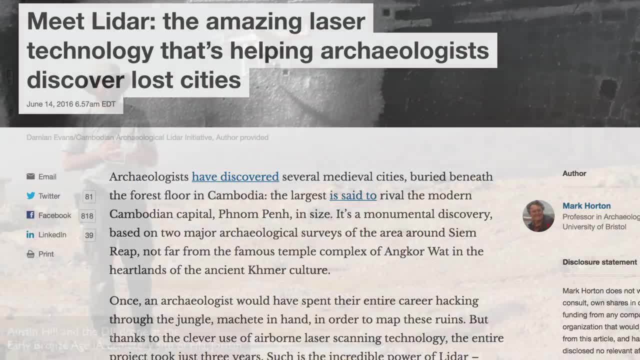 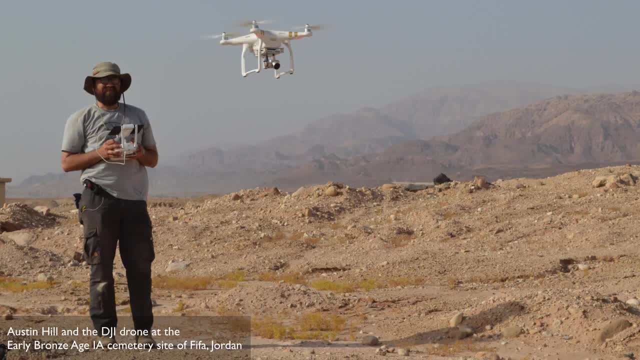 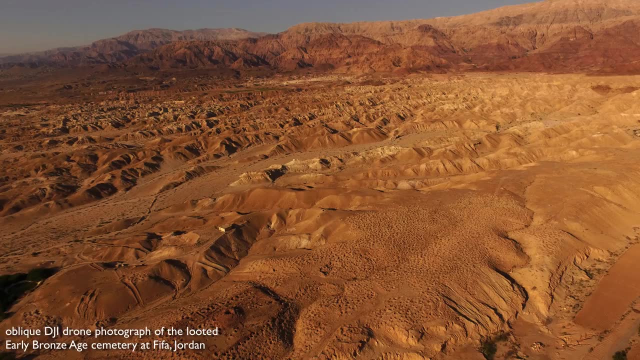 Airborne imaging, whether LiDAR or from drones or from fixed-wing aircraft, is further enhancing that. It's enhancing our ability to read human landscapes and to see the human activity that happens over time in any given place, as well as to establish patterns of human activity in the landscape. 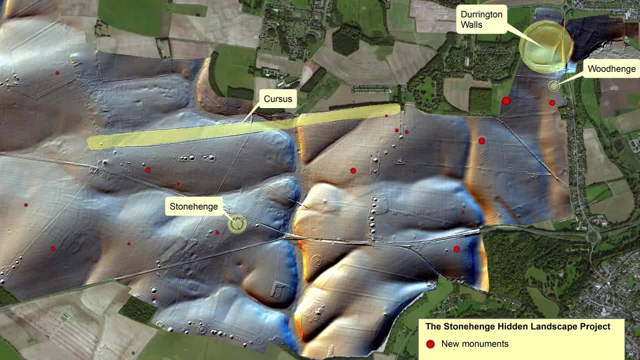 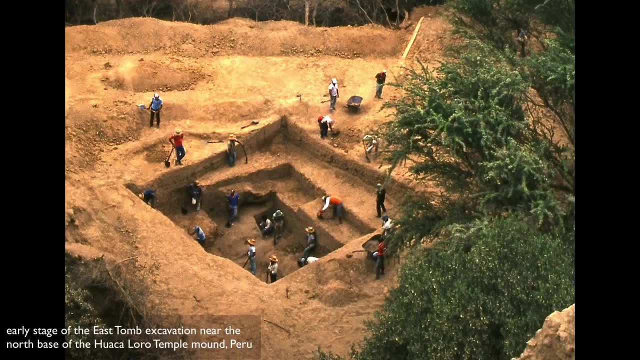 So not just focusing on a site, but seeing groupings of sites or patterns of human occupation in the landscape. Archaeology is always destructive. in some way One is undoing those layers of the past. We often say that archaeology is the unrepeatable experiment. 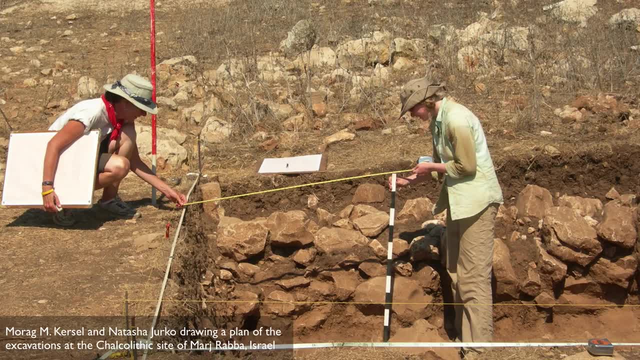 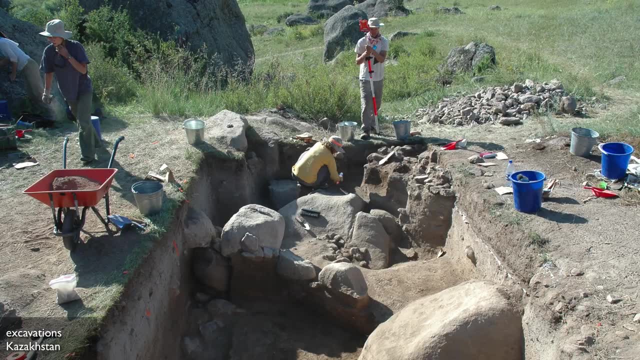 in that once the site is disassembled, there is no real way of assembling it. The properly conducted archaeological fieldwork is usually slow and maybe a bit boring, especially when compared to Hollywood versions of archaeology. But this slow methodical recording of the site, 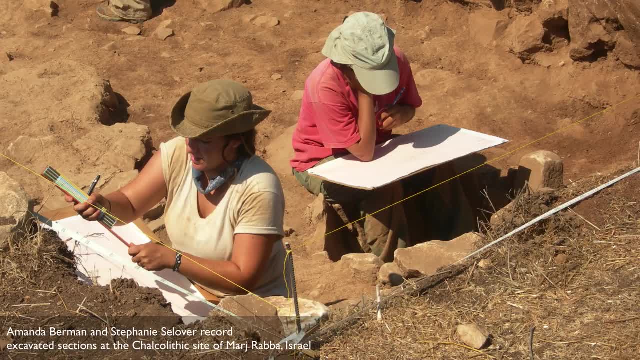 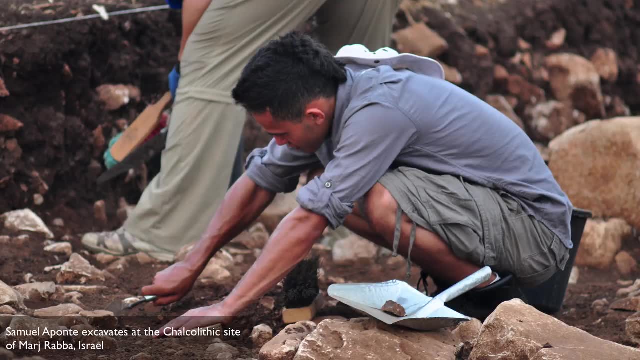 is perhaps the most important part of the archaeological method. But every site can only tell us a piece of a story. Any archaeological site, incredibly ancient or even quite recent, will always be incomplete. The archaeological record will always have gaps. One could even imagine that an archaeological site 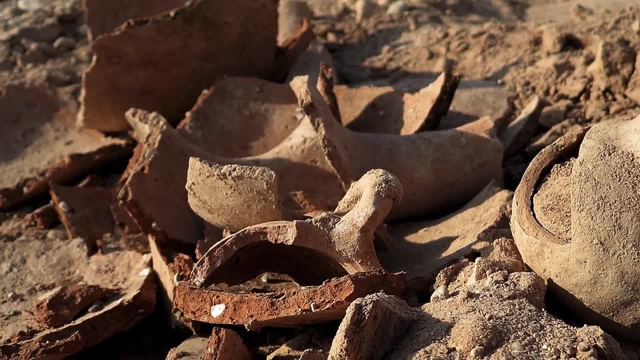 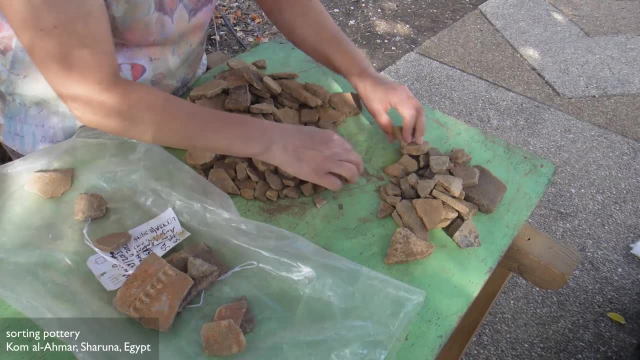 is like a 5,000-piece picture puzzle that one might have in the closet at home. only you've lost about 2,800 of the pieces, and that helpful picture on the box lid that shows you what it's supposed to look like has also perished. 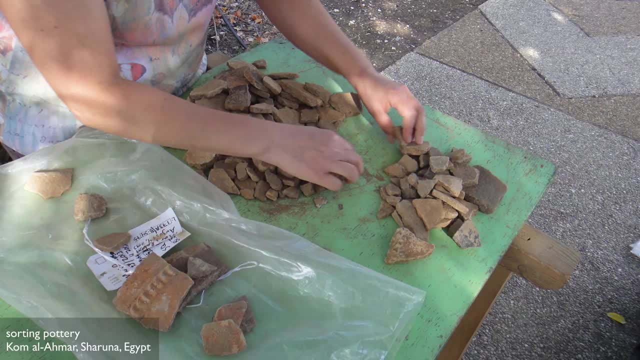 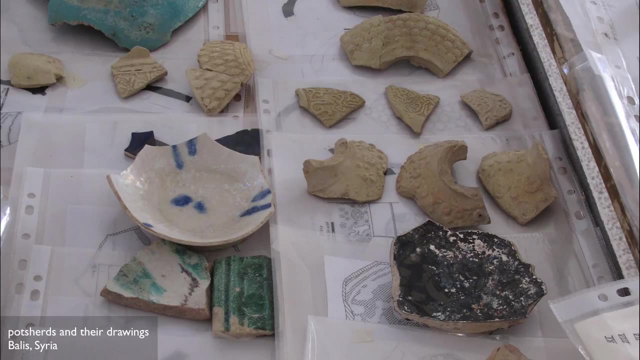 And so contextual interpretation means: can you use extant knowledge to fill in the missing pieces? And the sad answer is that you will never have a total picture of that place. but you can get pretty close, And that's why we want to do everything we can. 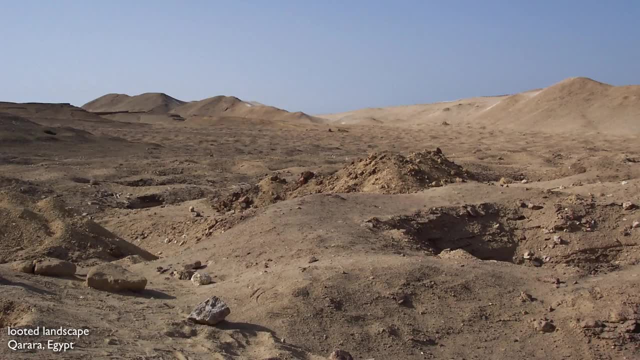 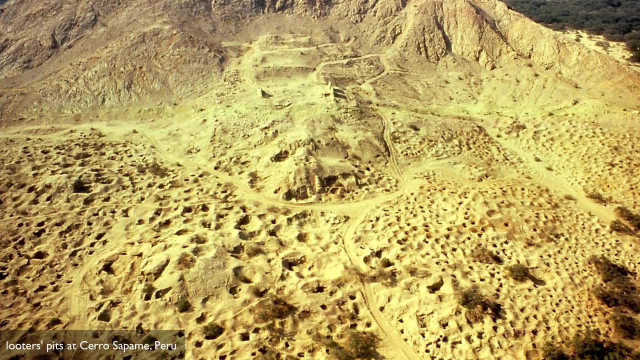 to preserve those contexts and discourage the destruction of archaeological sites through looting. Yes, we want to encourage people to think about the fact that archaeology is telling the human story And we need as many pieces of information as we can get our hands on.